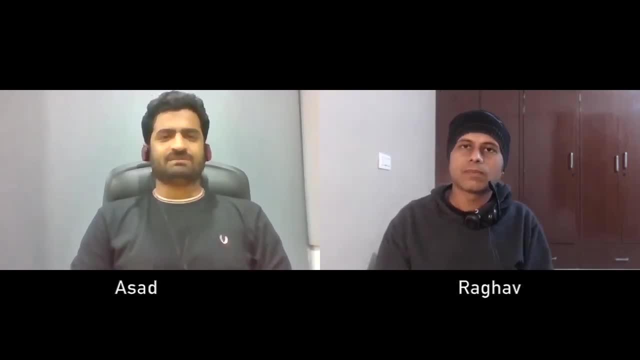 beginners. This is basically what security testing is, in a way. So I recommend you a type of non-functional testing that is performed to find flaws in security mechanisms and finding the vulnerabilities or weakness of software applications. Vulnerabilities like SSL pinning, injections, all kind of injections, denial of service, cross-site scripting, root port. 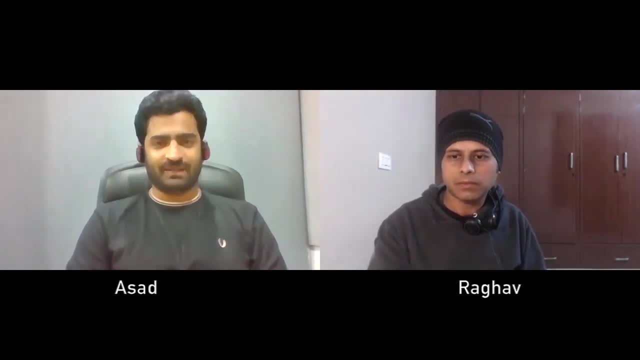 anything and many more. So security is an important aspect while developing a mobile or web application. It has to be- and it has to be- started from the initial level. when you are developing the application, You have to make sure that your code is secure and you do not. 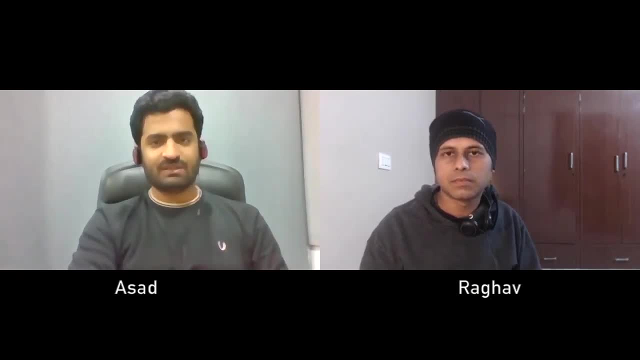 left any loophole behind. There are also tools available for this which ensures code quality and security, but irrespective of the domain of the application which you are testing, because the general perception is that security is only important for payments applications or where there any kind of financial transactions are involved. so they are very, very 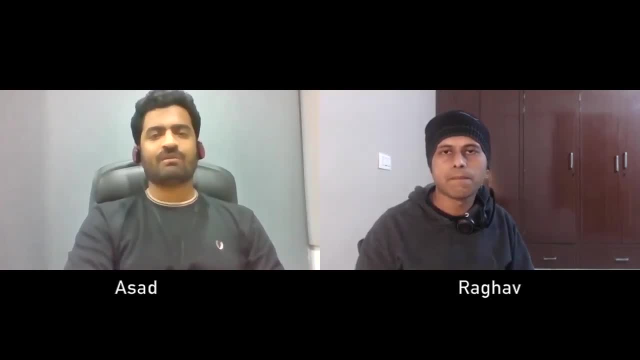 important these applications, but at the same time there are also strategies. but at the same time there are also also important for other general applications where no such financials are involved. so people usually relate security to a financial loss, but it is much more than that. uh. take data data leakage. 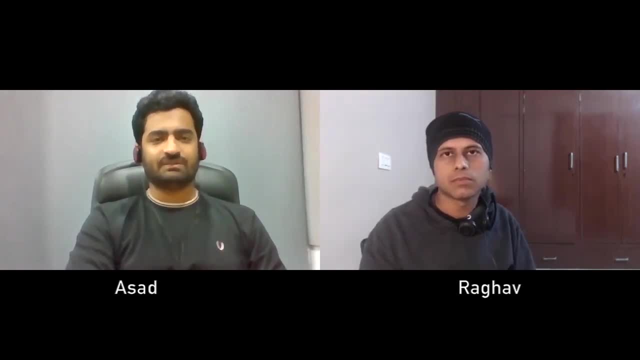 for example. it is a common example of a security threat that is harmful in any application, as this is the user's personal information that should be protected and must not be vulnerable to attacks. uh, it could be any sensitive information like the social security number, passport number, etc. 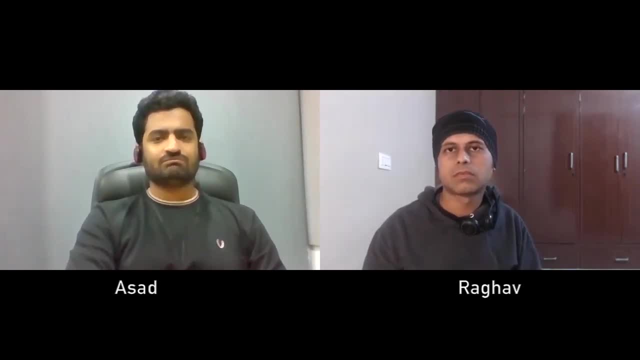 that in any way can harm the user. so, other than this, uh the responsibility, if i uh deeply talk about the responsibility of performing security, security testing, the responsibility differs in organizational, you know, in some cases it is performed by two engineers, some organizations, or throw it to any audit company as well, as they may believe that they do not have the necessary 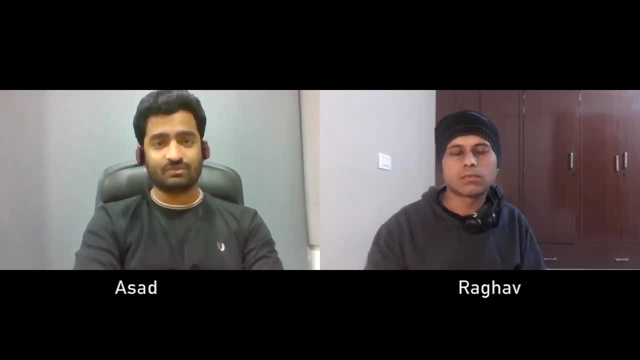 resources and tools to perform and they want to determine you test to be performed on their system. so they opt for any audit company and they provide them detailed technical reports with all the vulnerabilities, their severity, impact, sector, which helps them to resolve those issues. so yeah, in a nutshell, this is what security testing is. 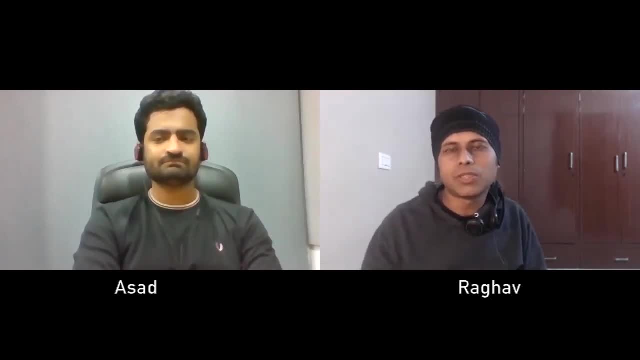 uh, great, thank you so much, asad. so, uh, you know, just to rephrase: uh, whatever you have said for uh, for the complete beginners on my channel, i will just say that, uh, we have functional testing and then we have non-functional testing. so functional testing is where you are testing. 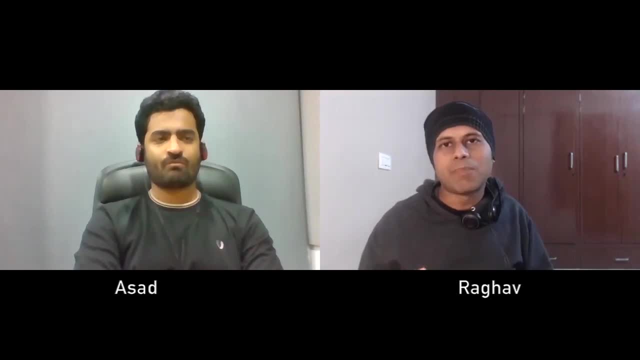 the actual functionality, the user scenarios. for example, you are testing a login scenario, so you will create a test where you will have steps to add or enter a username, enter a password, click on login and then see the result and you can have multiple sets of data: positive, negative. 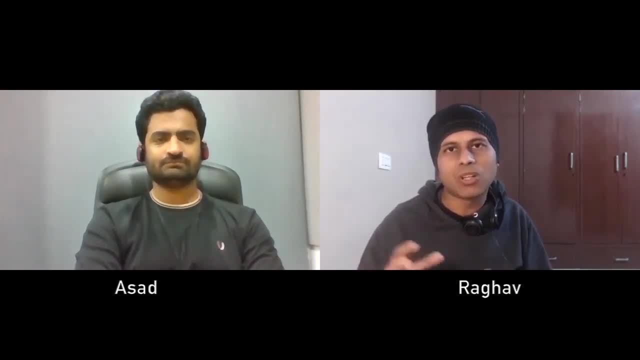 what happens when you enter wrong password or username. so all this will be a part of functional testing, but then we have no testing. where is where we test the non-functional aspects of the application and then performance, load compatibility, security testing. all these comes as part of the non-functional and specifically 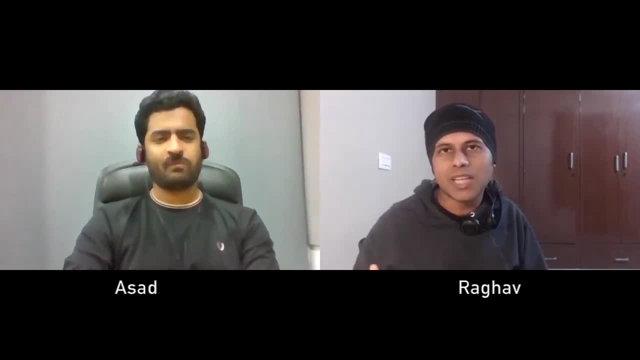 for security? uh, we check all these things that. how secure is the application? uh, is it susceptible to any vulnerability or attacks from hackers? and actually when we, when we do security testing or penetration testing, we check all these things that how secure is the application? uh, is it. 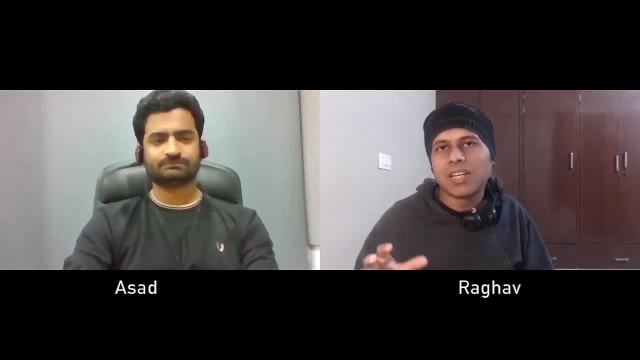 we actually try to hack the application. we, uh, work as an ethical hacker because we are permitted to do that testing, so we try to hack the application and see what are the vulnerabilities. uh, am I right or set anything to add here? Yeah, and we try to perform System. 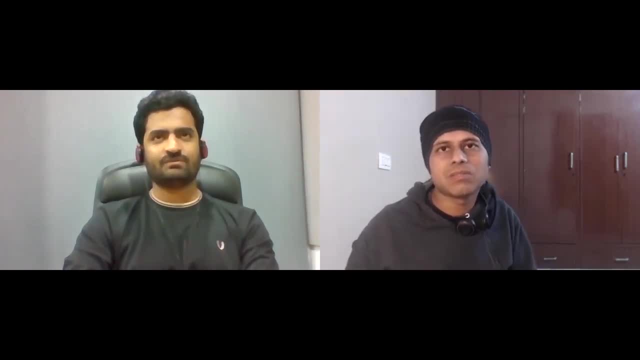 Fbud Rootो. up to what rush is virtual cloud firewall to become a hacking, but obviously in a controlled environment and with proper hedge event permission from all the stakeholders? yeah, exactly, exactly so. uh, that brings me to our second question. also, that is is a challenge. 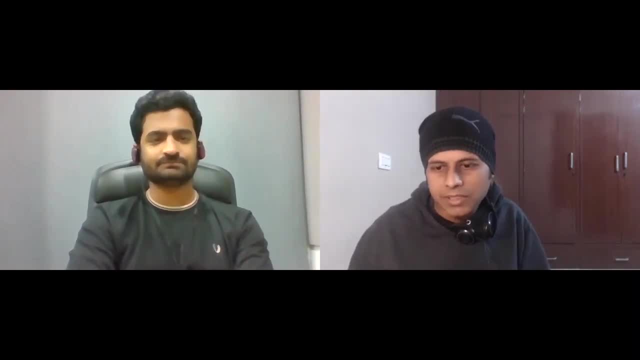 so we were supposed to write all the antibiotics or boosts. so, like we are saying back in the, That is for the complete beginners. I will just, you know, combine the second and the third question for complete beginners: how to start security testing and what are the tools, platforms and frameworks available, both licensed and free. 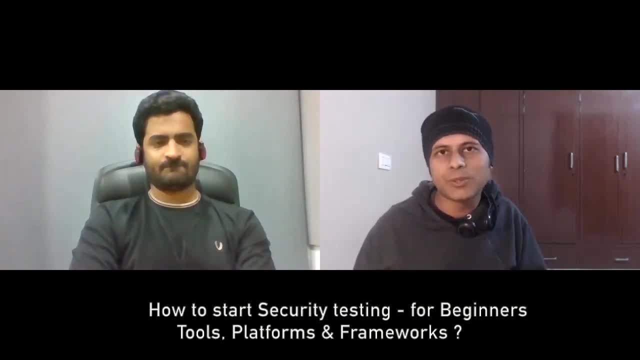 And I believe most of the people who want to start with will be more interested to know the free or the community additions first, so that they can, you know, start exploring and then go on with the paid tools. So how a beginner should start. what are the tools and platforms? 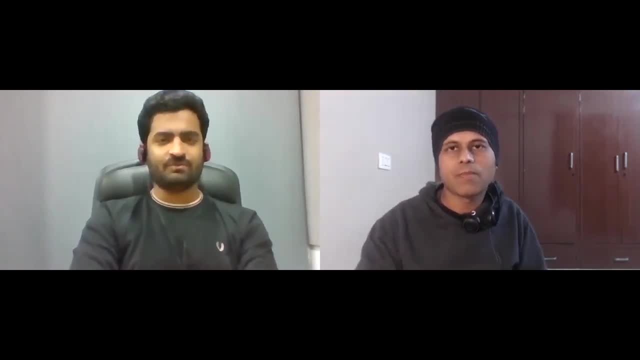 Yeah, if you are already a tester- obviously you should be- and you have a good experience in software testing, then you can also start with security testing as well. You should have basic knowledge of at least major vulnerabilities that you can exploit in all applications, in any application, like injection, gossip, scripting, DDoS, good code attack, all kinds of man-in-the-middle attacks, cell pinning, etc. 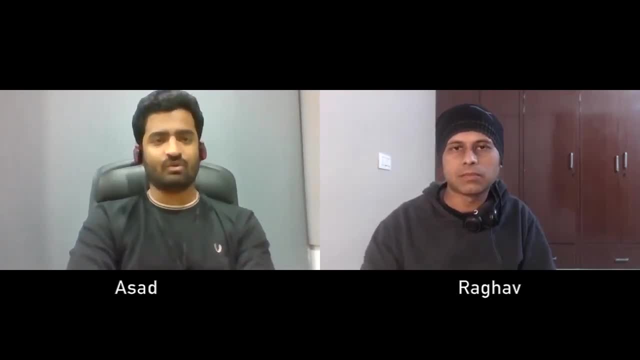 You can read and learn about these attacks and vulnerabilities on OWASP- OWASPorg- O-W-A-S-Porg. it is a very informative website and it can provide you a lot of information and useful information that you can learn, And you can also explore OWASP top 10 security skills as well. 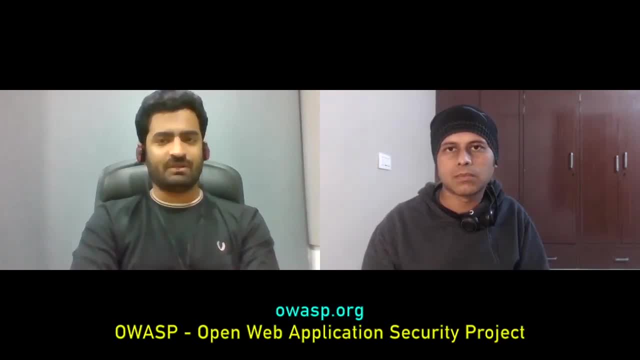 So sound theoretical knowledge of these vulnerabilities is very important. You cannot just glance and look at a vulnerability or attack on the internet and start exploiting it with the help of any tool, Every vulnerability you have to. you must have to understand this: that every vulnerability has its own impact. 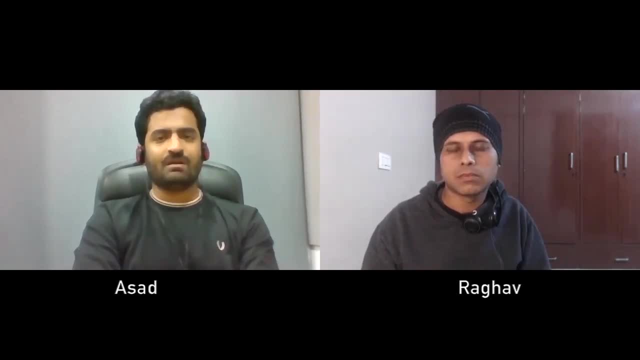 On the software, you should know the impact of the vulnerability, its remediation, its overall impact and its impact on your system. That is very important. So if we talk about a beginner, a beginner should start by looking at the URL of the website or of the endpoint that he or she is testing. 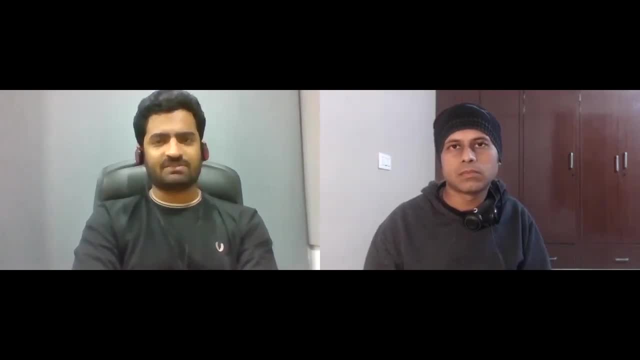 The one major aspect that ensures the security of any application is the HTTPS. Check if your website is transmitting data over HTTP Or is it transmitting. Start from learning the difference between them. I would simply say unsecured and secured. If you are using HTTP protocol, it is easier to breach the security, as data information being transmitted is in plain text. 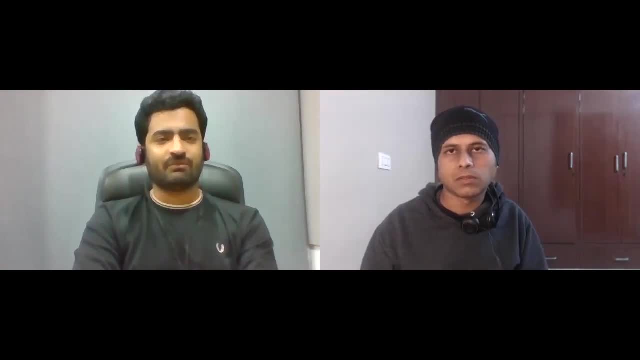 And the information sent is in print form. HTTP operates on application layer. HTTPS operates on transport layer- TLS. No certificate is required in HTTP. On the other hand, HTTPS uses TLS. TLS is a certificate to ensure authentication. HTTP is subject to man-in-the-middle attacks and eavesdropping attacks. 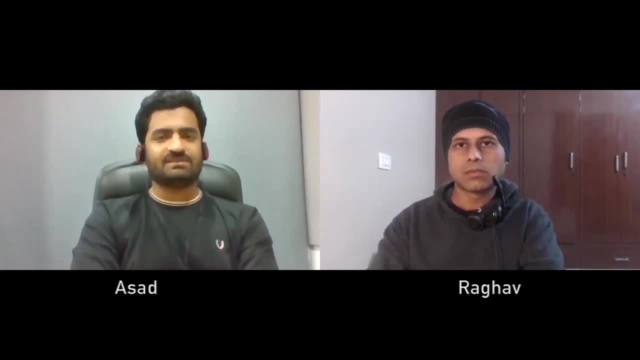 HTTPS is designed to resist these attacks and is considered secure against such attacks. You know the S in HTTPS is secure socket layer, SSL. It takes care of ensuring that the data goes securely over the Internet. This made man-in-the-middle attack increasingly difficult, as the data sent is no longer in plain text. 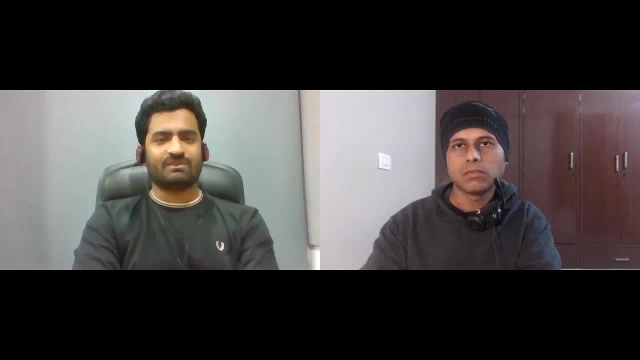 But that doesn't always mean that we cannot temper any request or response and eventually perform a successful man-in-the-middle attack. We still can if SSL pinning is not implemented. Now we can discuss what SSL pinning is in this session as well, or in upcoming sessions, as you want to proceed. 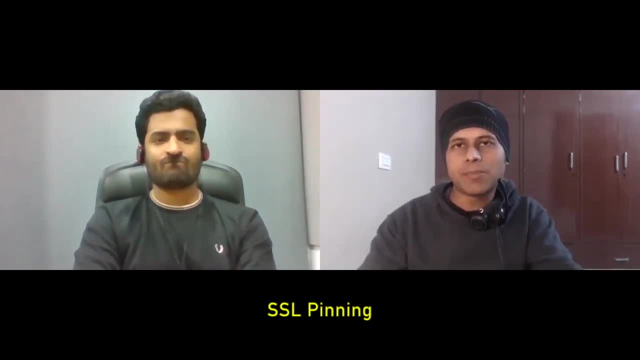 Yeah, Asad. So I think you know we can keep this session very basic and then we can take this conversation and discussion forward in the coming sessions where we can take up, like SSL pinning or you know specific terms and technologies related to security testing and all those things. 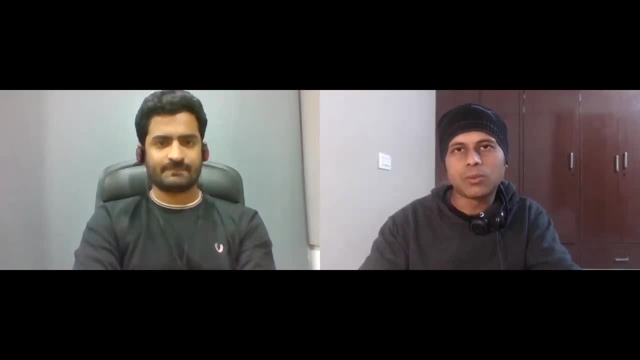 So I think this is good for a beginner to start to you. You can you know very, very basic thing is you can start looking at the URL of your application. If it is a web application, then does your URL has HTTP or HTTPS? 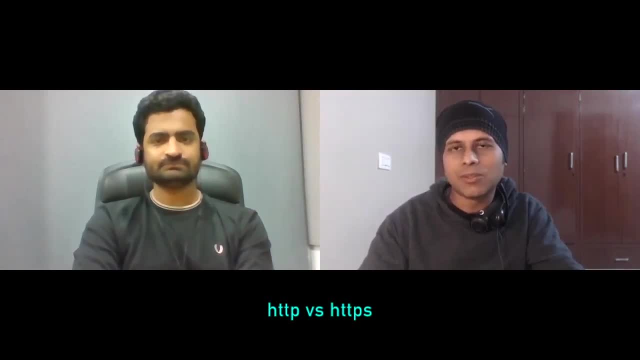 S is the secure part. So you should have the- you know HTTPS URLs with all the certificates And all these basic security things And then you can go forward with the with the deeper levels of security. So that was very useful, Asad. 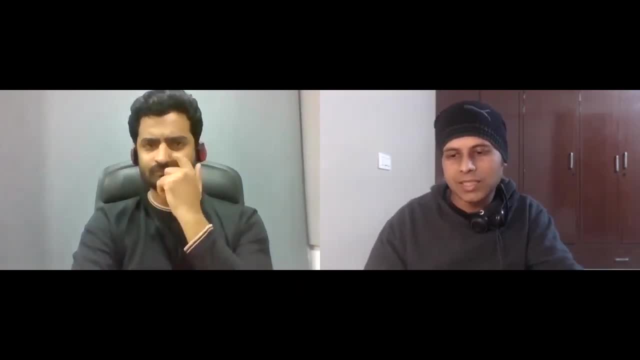 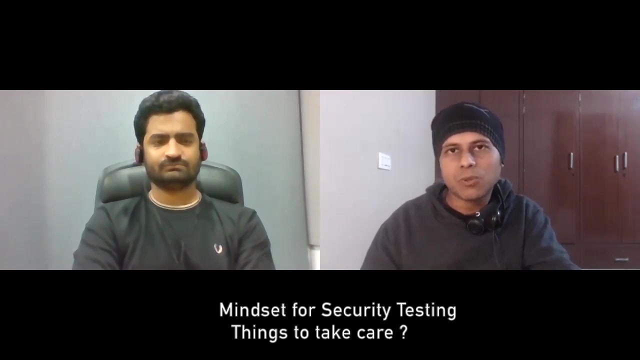 I think the next two questions again we can combine. that is, mindset for security testing. What should be your mindset when you are actually trying to do security testing And then what are the things to take care? Now here, with my experience, I can say that whenever you are doing any kind, 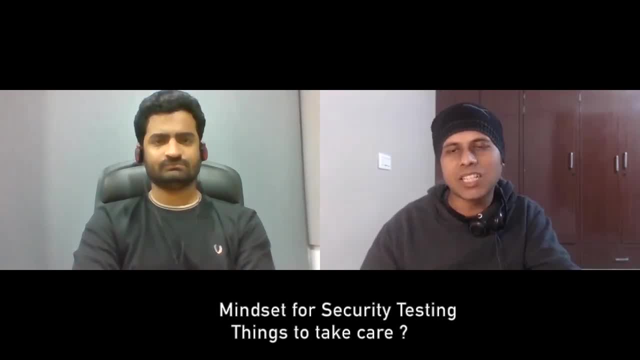 Of security testing, you are actually going to hack the application as an ethical hacker. Now, if you are doing this- you are you are doing to hack some application- You have to be very, very careful that you take a written permission from the owner of the application. 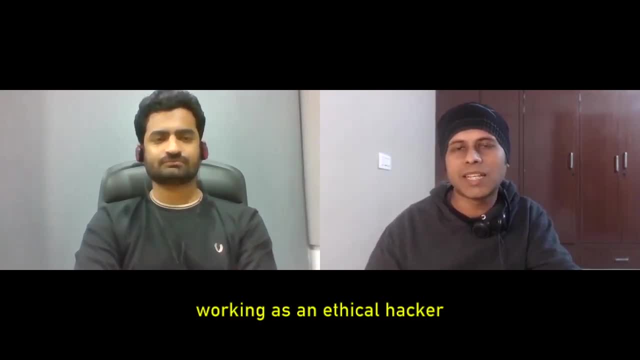 Or if it is your client or a product manager. whoever has assigned you the permission or authority to go and do security testing, You should always take a documented written permission that you Are Allowed to do security testing on this application, and then you should also be having complete awareness on what parts of applications you can go into and do the security testing or penetration testing. 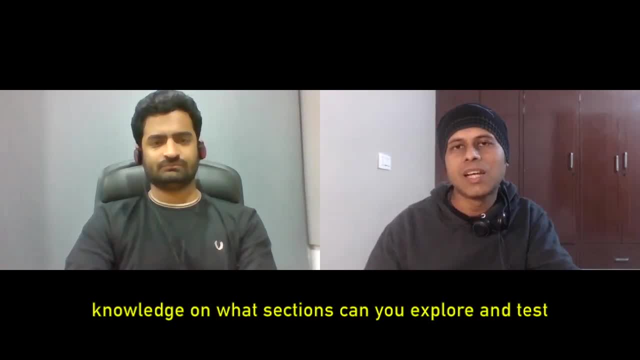 So again, you should, you should document it, take permission on that, And of course you should do it on a controlled environment. So I said I think anything to add here. what are your thoughts on the mindset and things to take care? 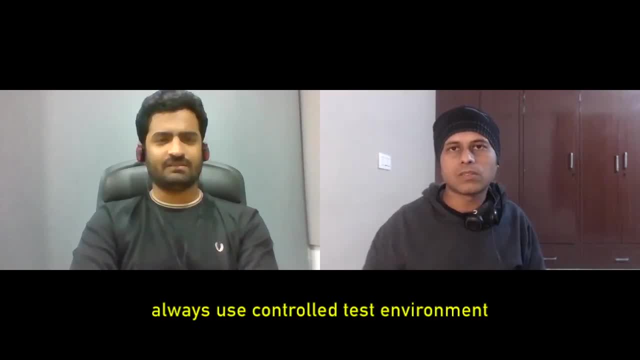 Yeah, before coming on to that, I've Just like to add a little informative thing on the tools a beginner can use and explore at this stage. At this stage, I would recommend one tool for the beginners. that this burp suite. burp suite. 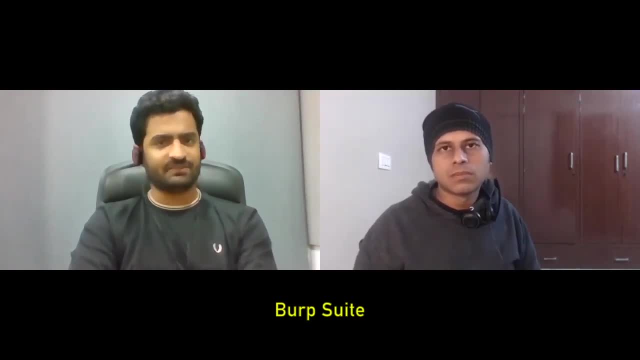 It comes in two editions. One is community edition, That is a free one, And one is professional edition, That is the licensed version and community edition. You can perform most of the attacks, mostly manual. that will cover major testing of your application. I personally use this most of the time. 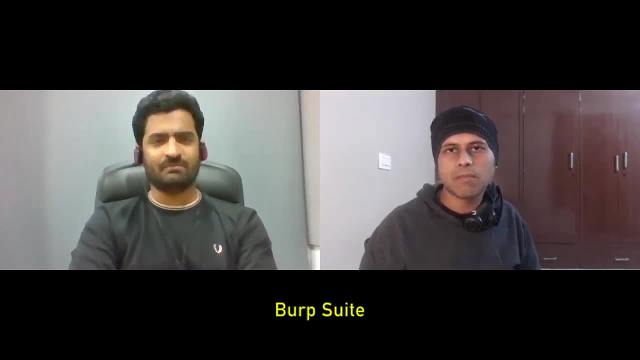 It has a repeater and Intruder, interceptor, sequencer, compare or everything that is required to perform security testing on any application. On the other hand, there's a professional edition which comes with a scanner- built in scanner- which scans your application and looks for vulnerabilities and give you a comprehensive report which unfortunately doesn't come in community edition. 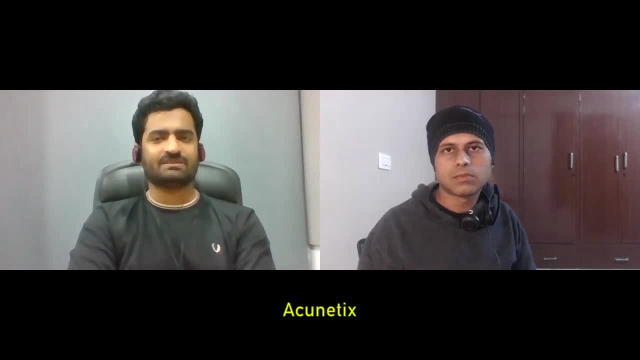 There is. then there is Acunetix, which is basically a scanner which I think comes in three editions of your standard, which is the free one, premium and Acunetix 360.. Standard, obviously, is very good. It's very good. 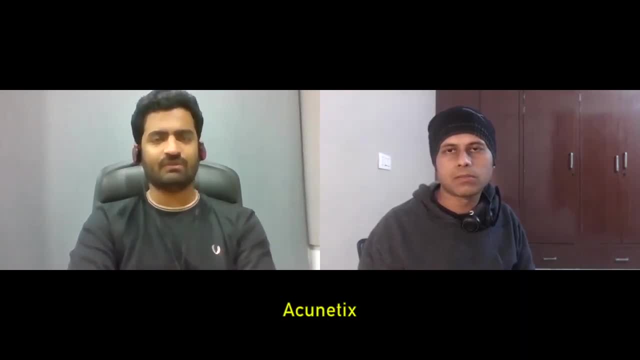 Obviously it's very limited features, but it can still scan your endpoint and give you all the phone vulnerabilities with its severity and remediation. It is installed as a service in Windows and runs on your browser. Then, on the third, we have also has OVAS Zap, which is again a good security testing tool in which you can perform almost all kinds of attacks quite easily. 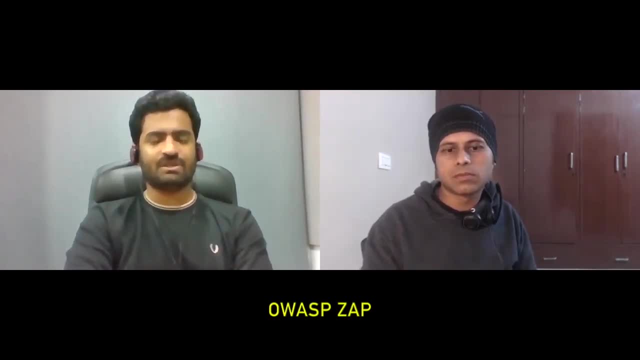 And it is also open source. I recommend this after burp suite. So there are obviously some other tools as well, like Kali Linux, etc. Which will look into a. So, coming back on to the, to your question about that thing which we need to take care of and performing, 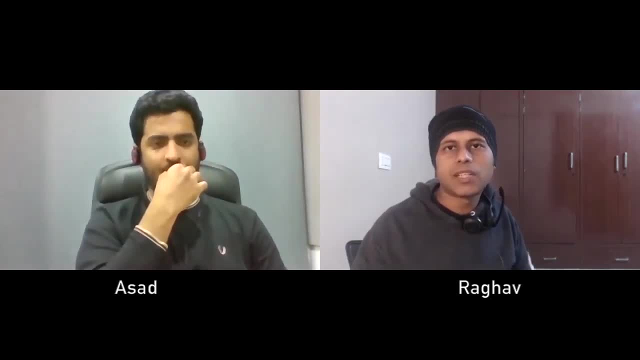 I said before going there. I just want to make sure that the three tools that you have recommended is Bob suit, and Bob suit has a community edition so people can start using it free on the community edition. Then we have Acunetix again. 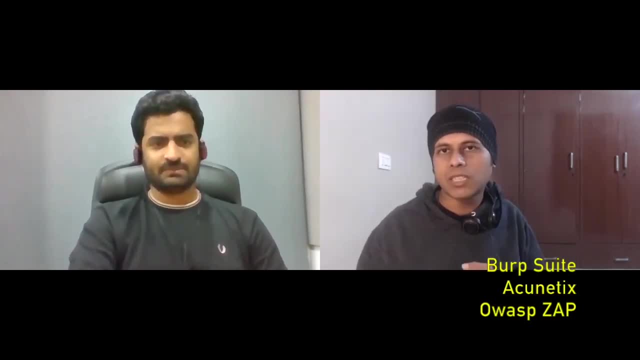 Acunetix has a free community edition. and then OVAS- OVAS lab, Again, it has a. it has a community edition. Right, Yeah, it's open source. Yeah, great, So, great. So these are the three tools that you know you can start exploring. 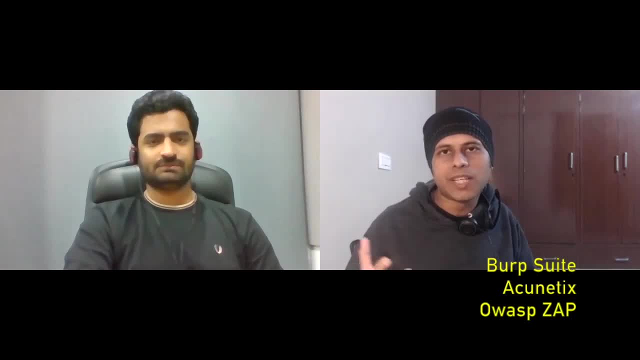 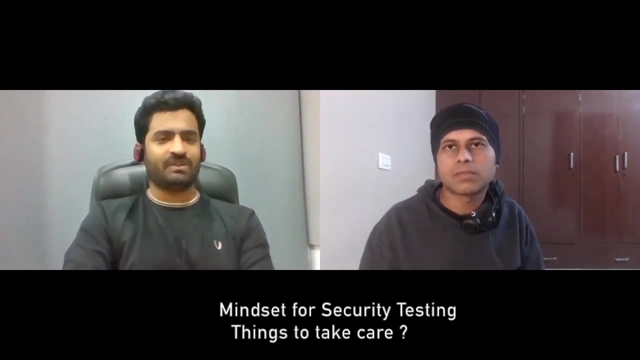 You can start looking at tutorials and then you can start using them, So this will be very useful. Fine, Asad. So let us go to the mindset and things to take care for security testing. First of all, do not start exploring and using tools without proper knowledge of security testing concepts, vulnerabilities, attacks and their impacts, etc. 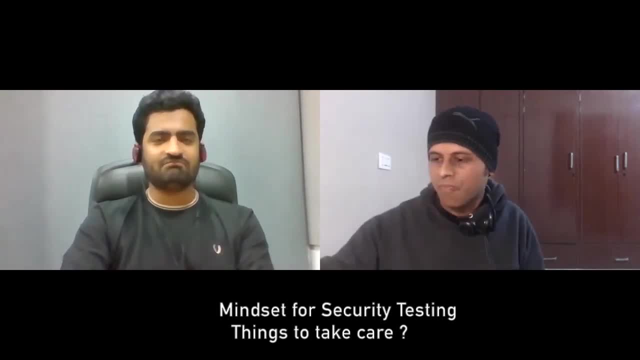 As I mentioned, As I mentioned earlier, you cannot just read about vulnerability, not understanding its impact, its remediation, its overall impact on the system. You cannot just go and exploit it on any application. You do not have to do that and do not test, pen test, any application without proper written permission of all stakeholders. 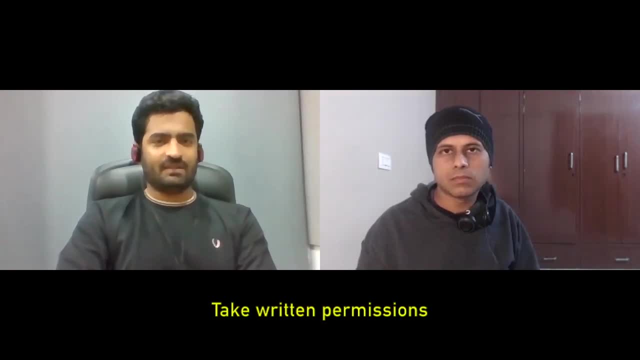 You do not want to be unethical at all at any stage. Next, always perform all kinds of attacks in a controlled environment. You know you can. If you, if you, if you can, you dedicate a separate machine for this. do not use the dummy. you do not use actual live accounts for testing this. use dummy data, create dummy data. 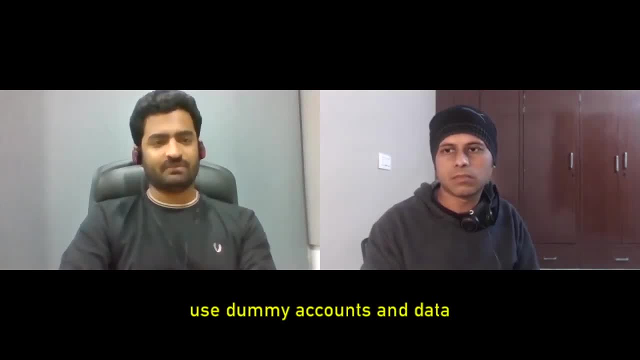 If possible. if you have a lab set up in your office, it is, it is great. Perform it in the lab. perform it with proper permission by giving a heads up to all the stakeholders. set up the environment or any server that you need to prior to performing any activity. 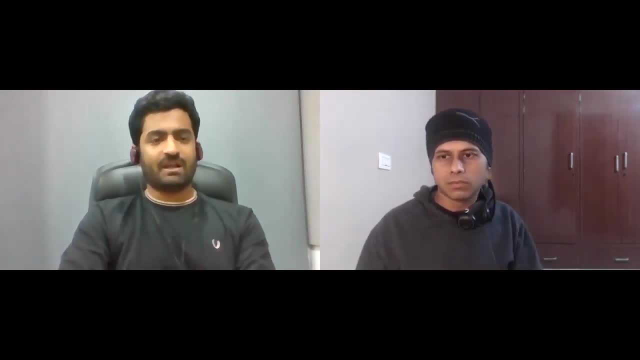 Great, Great. So it is very important that you take a proper notice before performing any activity. And, again, if your application uses some third party services, you should also take them into confidence that we are going to perform this on your cloud service or whatever. 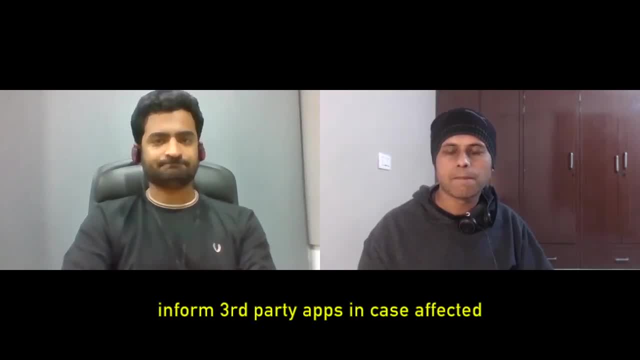 And so they, so they must be aware of your activity. Yeah, That are very valid and great points. Remember, whenever you have to start with security testing, make sure that you have authority, you have authorization and you have the knowledge to follow all the requirements that are required. 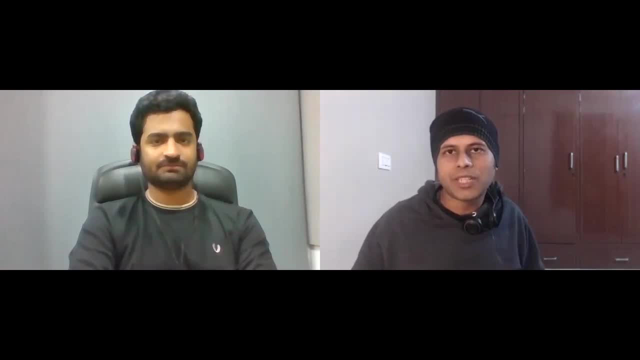 If you are an Office 365 user, you should have security checks, And the security checks are the ones that you have to follow And the security checks are the ones that you have to follow. You know, if you have to follow all the requirements that are required for the security tests, you should follow all the requirements. 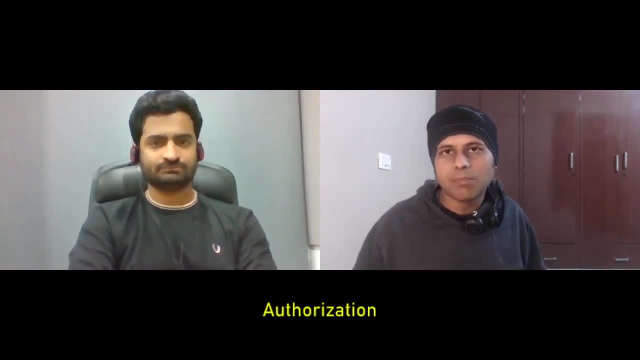 But if you are an Office 365 user, you should also be aware of the instructions. you have authorization or written permission to do the security testing or penetration or pen testing, as we say for on the applications from the owner of the application or your product. 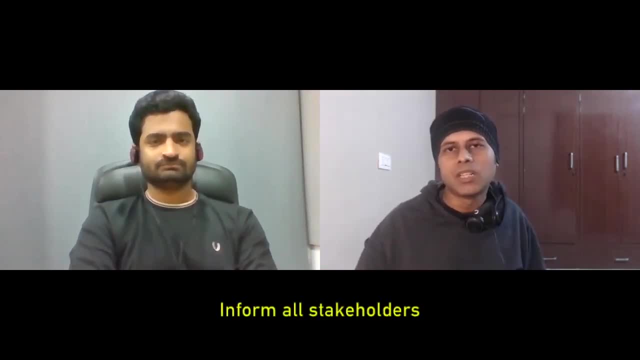 management team and every, every stakeholder should be informed. and i think the other important thing is: whenever you are trying to learn security testing- and you are trying to do it on any application- you are trying to hack an application just for learning security testing. always use some dummy apps and some dummy accounts. do not start to do security testing on your facebook. 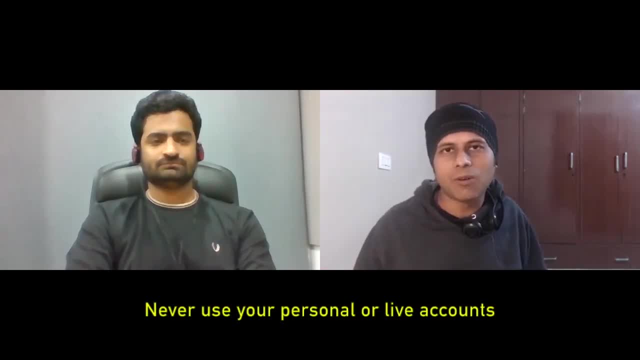 primary account. you will end up deleting or deactivating your account and then there will be a lot of damage. so always use some dummy apps, some dummy accounts and again, try not to do any kind of hacking or security testing from your personal machines, laptops or computers. 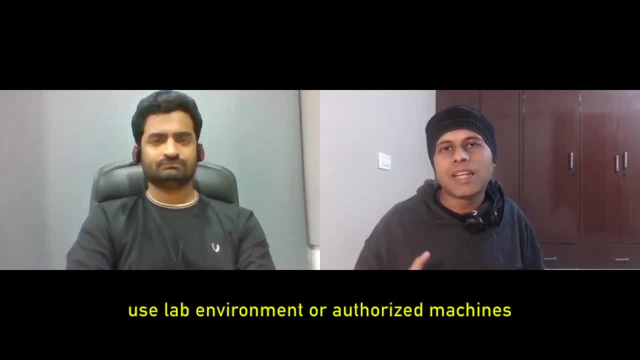 always have some lab or some remote systems and you you can, you know, create some remote systems like on aws or any other cloud services, so that, even if something goes wrong and you have to actually deactivate or let go of the entire system, it is fine. so we these are some very, very important tips and things to take care for: security testing. 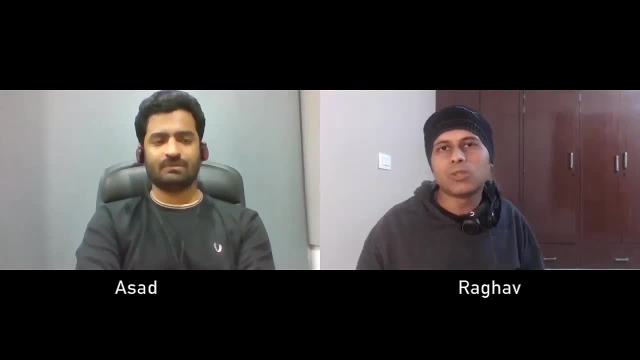 so always do it on dummy apps, dummy accounts, and also use some remote system, some other you know system, which are designated for this activities- am i right asad here? obviously 100, great, great. so, uh guys, this uh session i wanted to keep it very, very basic and 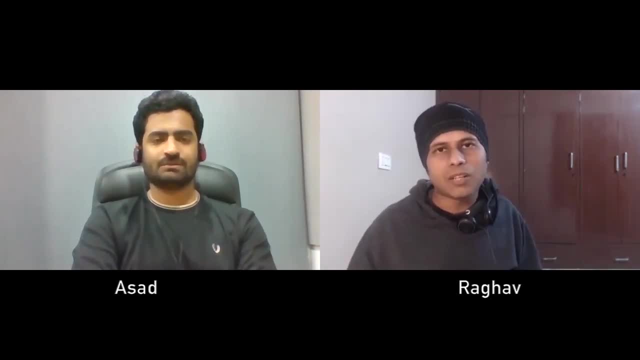 simple for the complete beginners who are yet to start on security testing, so that we can get some very basic things and points, so that we have these things in our mind and we can take care of all these points while we think or start of security testing. i will try to have more sessions, uh, on 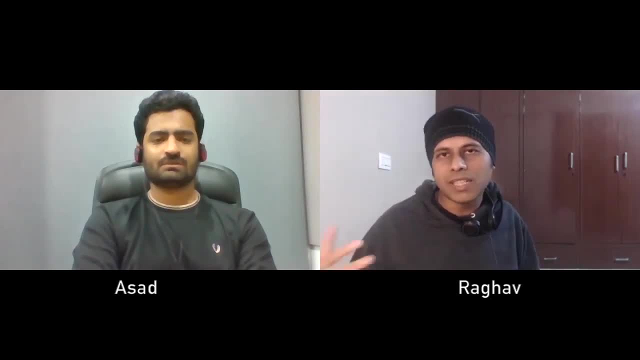 security testing and discuss on more, uh, you know, intermediate and then high level things and go a little more deeper into security testing. but yeah, this session, uh, we are going to have all these, uh, basic stuff so that you get some basic knowledge for starting with security testing. so one of the important things that we 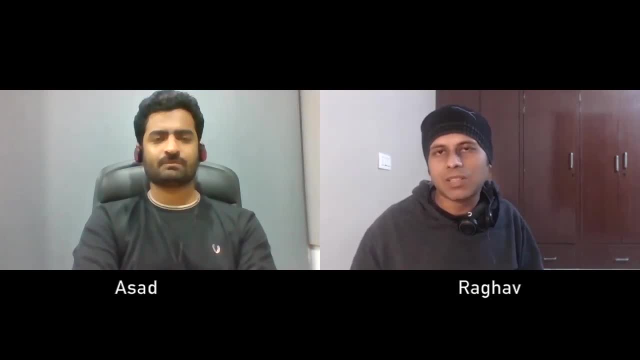 discussed today uh was how to start with security testing. uh, what? what are the basics? what is security testing? the tools that you can start free of cost? uh, you can start with the community edition. and then what is the mindset? what are the things you should take care while starting with security? 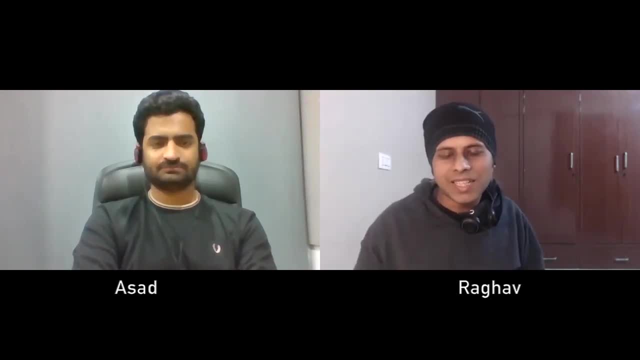 testing. so, asad, any any other general tip, anything else you want to add before we wrap up this session? yeah, i'd just like to add some uh tips for your for the mindset required for security testing. like, think like malicious hacker, you know, make uh, let your brain a little detective for this purpose, for. 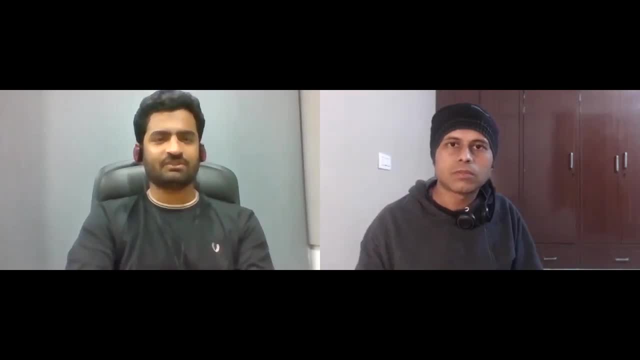 this. you don't need to study or learn anything but other. you will explore and develop the ability to explore it. as if you want to add some of these bits and pieces as well, alright, good, thank you so much. uh, any application yourself, if you just start thinking like a hacker or attacker. so when you 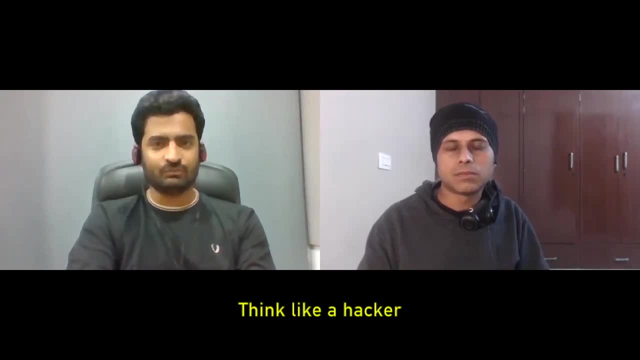 do this, you will automatically search and explore different techniques and tools you can use to automatically search to find and exploit major vulnerabilities. you will find vulnerabilities in validation messages and even in the application flows as well. let's take a common example when you log in an application, a valid common example of a validation message when you 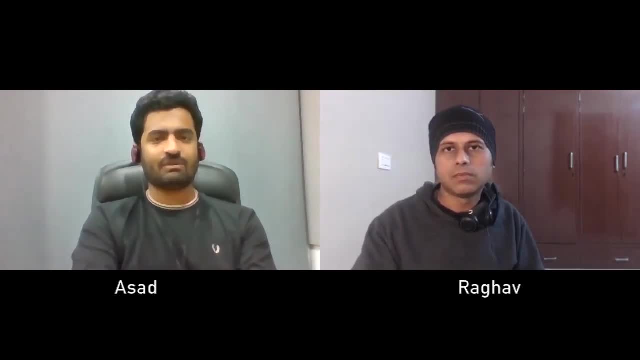 provide valid email address but invalid password and see what validation message appears. if it is invalid credentials, then it is fine in terms of security, but when it says invalid password, then you as a pen tester or hacker could easily see the vulnerability in this message. giving invalid password error means that the user does exist with this email address, but the 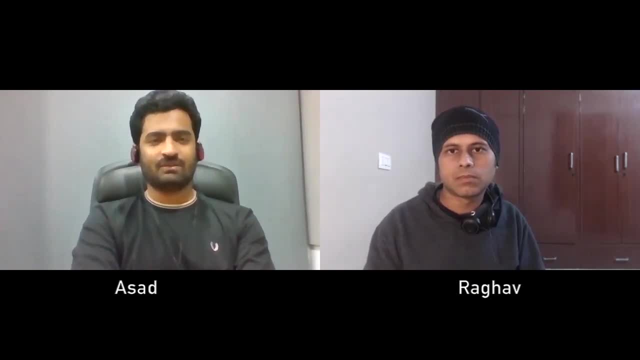 password is not correct. so you find this vulnerability in the system. now the next step for you would be to to exploit this vulnerability and actually use that email address to guess password of that account by attempting multiple logins with different passwords. ahead and try a technique, and in pen testing we call it the brute force attack. 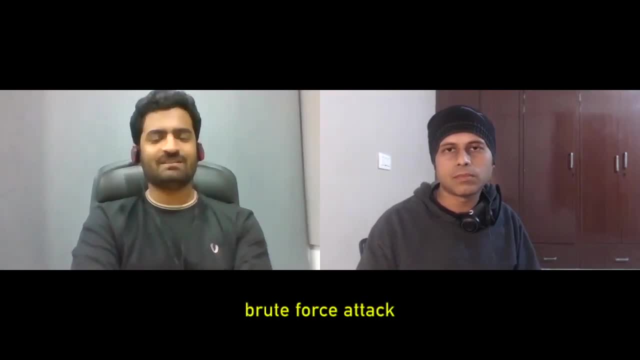 so you see how you managed to find the vulnerability and ultimately explored it through brute force attack, and you learned one of the major techniques through which you can take over any account. then, at the same time, you should be- at least you should be- that much equipped with these concepts that you should not be. you should also be. 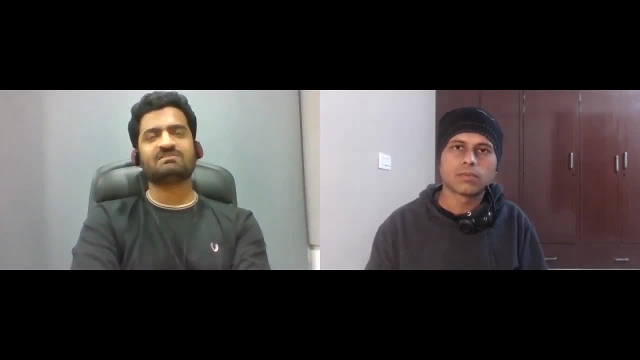 able to suggest remediation for this vulnerability, like you can suggest that to prevent brute force attack, we can implement account dropout feature or two-factor authorization. you know, capture every request and response, try to perform all kinds of management attacks. one more thing: you should also enhance your analytical skills as well, because it is a very important security testing you should. 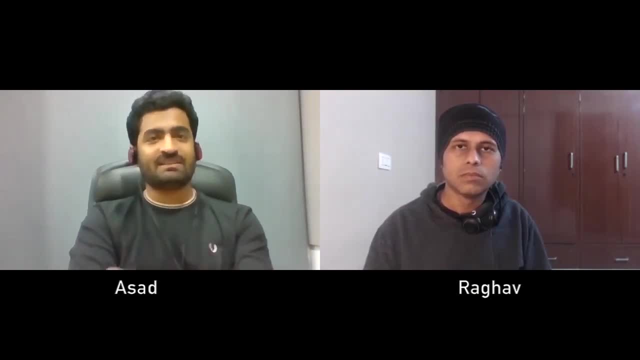 be able to analyze requests and responses, uh, and, like the pattern of encryption, passing of data for one response to the other, uh, analyzing the parameters, you will then be able to exploit more vulnerabilities. believe me, let me give you, we can uh keep this example for the next session. yeah, 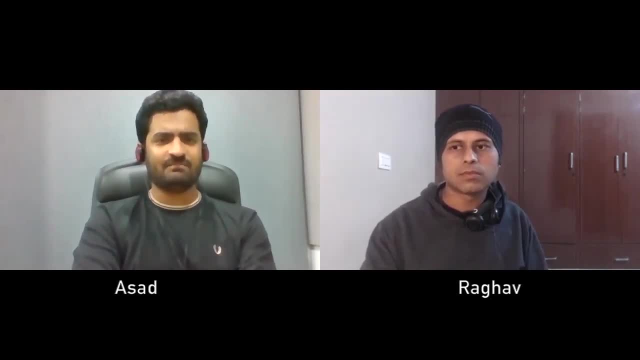 but analytical skills, analytical skills and uh, thinking like malicious, like that- is very important when you're performing security testing. yeah, asad, i i know you know being into security testing, you might be having a lot of examples and some some uh really good examples and some uh very interesting things that you can, you know, share with us. maybe we can have our next. 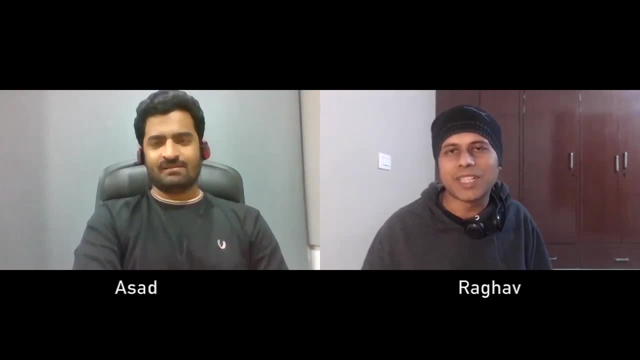 session where you can share all your interesting experiences with security testing and, uh, you can give some examples. uh, i i can think of. you know one um one of my experience that i was doing security testing. we were into an organization and i was doing security. i was actually doing. a functional testing of apis and uh in the. in the response of one of the apis- suppose if you give some wrong information, it was giving a response that the connection with the database could not be established, and it was in the response message. in the error message it was also saying what is. 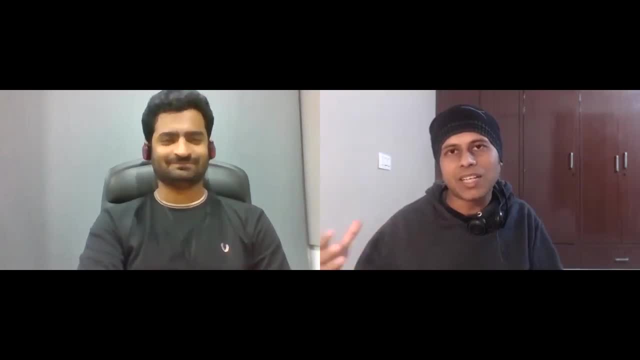 the database. it was oracle. connection with the database, oracle xyz, could not be established. so you should take care of these things: that your response should not tell the user what is the database or what is the backend systems you are using, because with this you are taking the hacker. 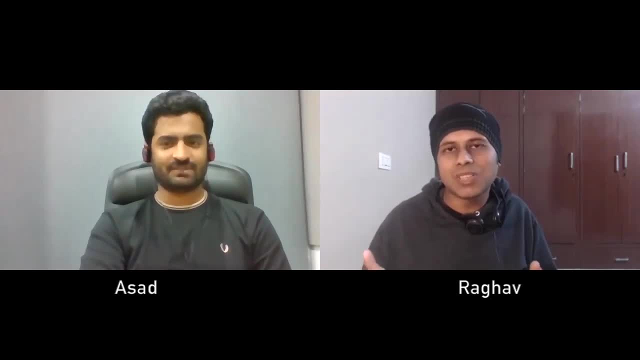 one step closer to hacking your system. so you should always take off these very simple things- that are my responses, or are my error messages, giving out some information about the backend systems, about the tools or anything that we are using. so i think this is also, you know, one of the good examples i can think of from my 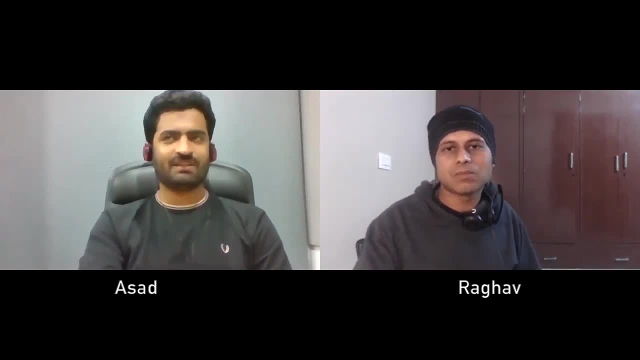 experience. yeah, exactly as i mentioned. look for the level of information disclosed through your application. information disclosure is yet another vulnerability in security testing. as you mentioned, look for security headers and information in the system so you can look for security headers of the request and response and then, at the same. 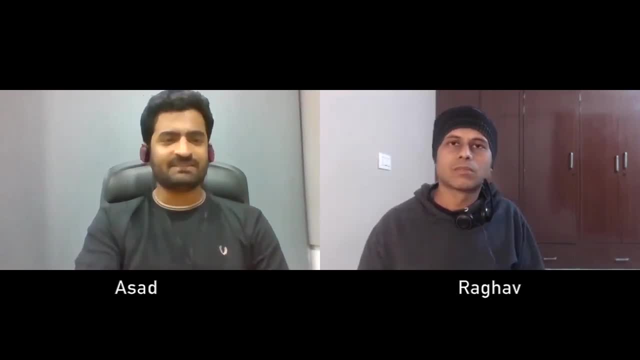 time. you must be good at api testing as well, because most of the time we can observe, intercept and temper these api requests and responses to the system. so, yeah, adding this to your point. uh, great asad. so it was a great session and i hope all of you have got some good inputs to you.